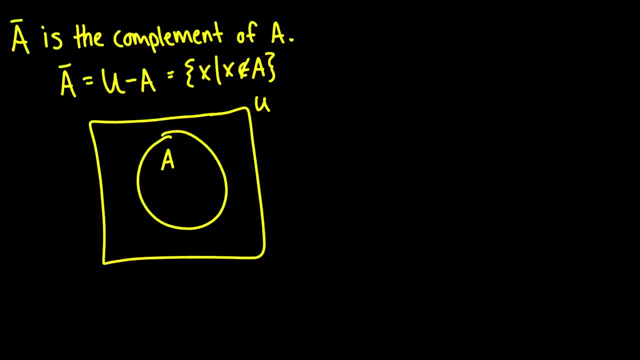 couple things here. We can talk about the complement of a set and we define the complement as everything in the universe that is not in A. So if we have a little Venn diagram here and we color in the complement of A, what I'm shading in is all the elements in the complement of A. So basically, when we have this, 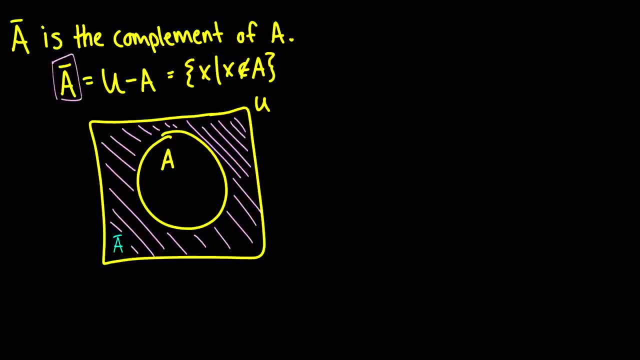 A bar. here. we're just talking about everything, not in A. So if we have A is equal to Z plus and U is equal to the set of integers, then A complement is going to be the set of all negative integers, Because we're just taking: okay, well, the whole universe is the integers and our set, A, is going. 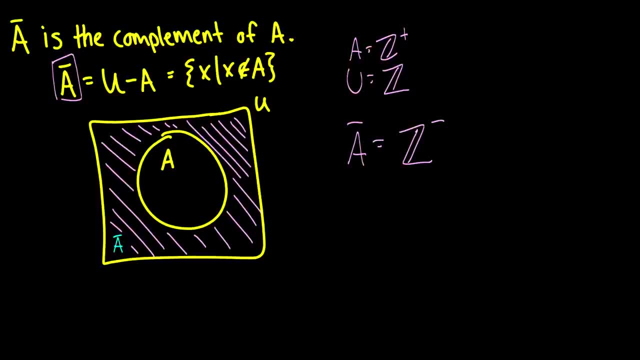 to be just the positive ones. So everything that's not a positive integer then must be a negative integer. Therefore, this is the complement of A And this is denoted A bar. It is sometimes written as A prime and sometimes written as A complement, with a superscripted C And, of course, in set. 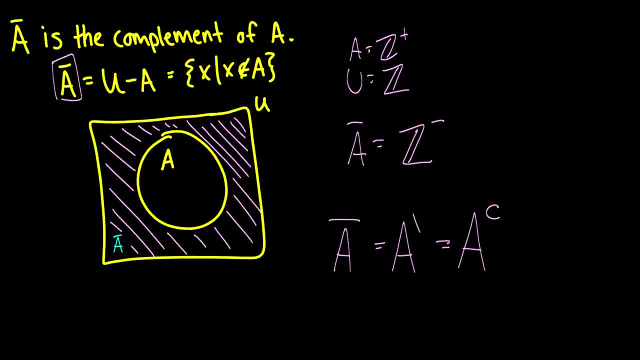 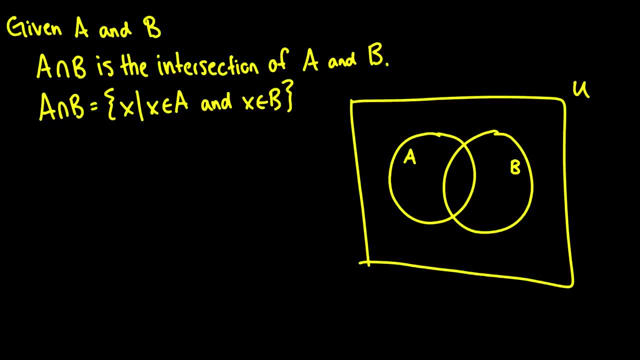 notation: this is the set of X, such that X is not in A. We can talk about intersections. So now, if we have two sets, we can say: well, what is the intersection of two sets? And that is going to be everything. 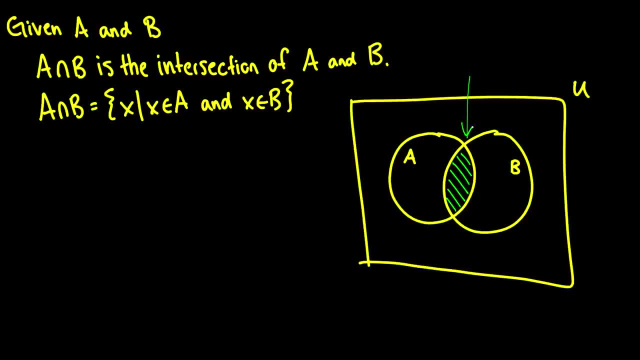 that is in both sets. So we write this as A intersection B And it's kind of like an upside down U. So this is the set of elements that are in A and also in B, So in a Venn diagram. well, 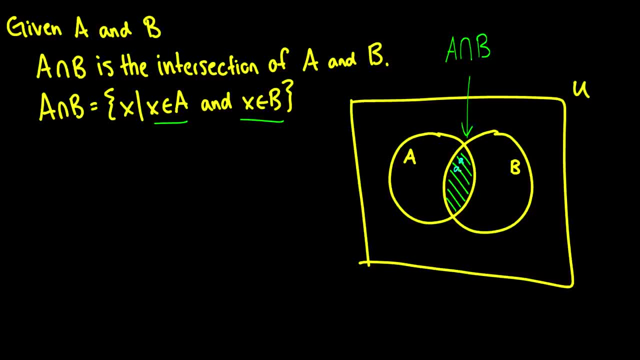 here, where we have our little A's and we have our little B's here, and they're both in both sets. So we call this A union or A intersection B. So if we have B is equal to 0,, 1,, 2, and we have A. 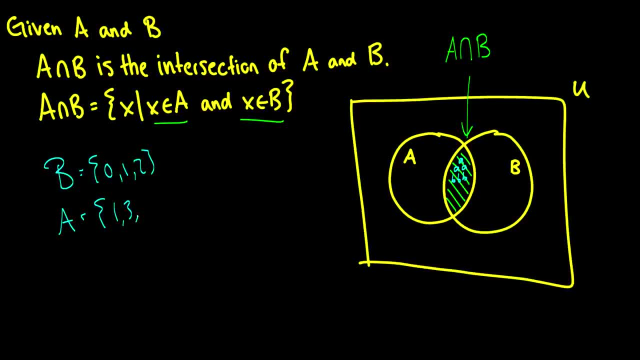 is equal to the set 1,, 3,, 4, then things that are common in both sets. well, we take a look, We say, okay, is 0 in A, No, it's not. Is 1 in A? Yeah, okay, So both of these are in both sets. 1 is in. 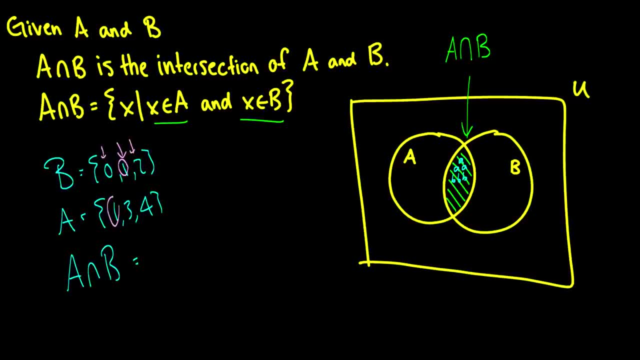 both sets. What about 2?? Nope, Okay. well then, we have our intersection here, which is just the set containing 1.. And if we wanted to draw this here, we would write: okay, well, 0, sorry, 3 and 4 are in A, 0 and 2 are in B and 1 happens to be. 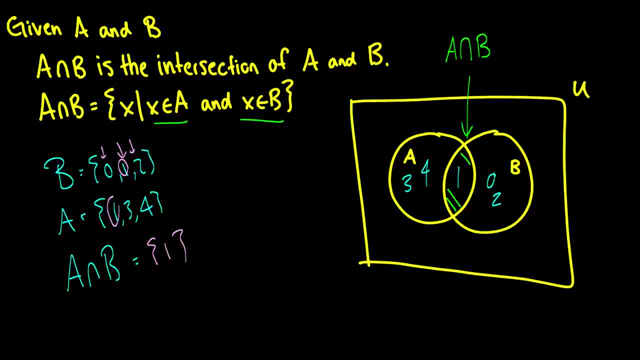 in both. So if we were to extract these sets out and take a look at just A, we would see 3,, 4, and 1.. And if we were to take a look at B separate, then we would see 1,, 0, and 2,. 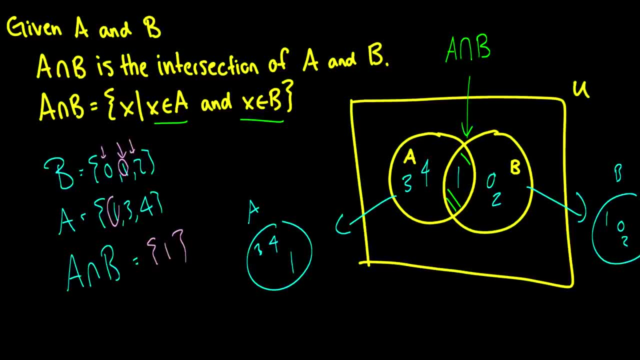 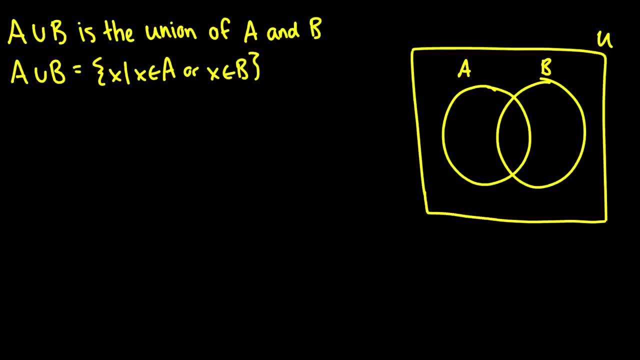 which correspond directly to the sets we just looked at. Here we have A, union B, which is the set of things that are in A or in B. They can be in both if they want to be in both. So basically everything here. So let's say we have A- is equal. 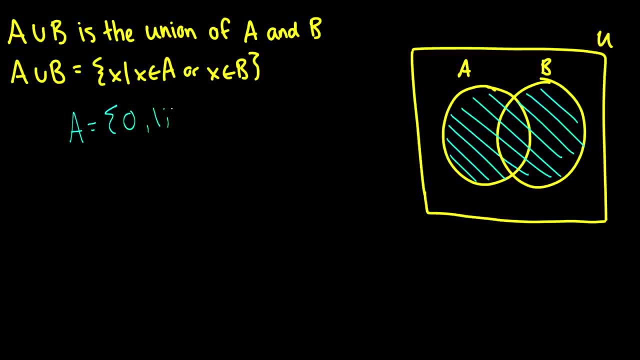 to. let's take the same things here. Well, I'm going to switch the letters around: A is equal to 0 and 2, and we're going to say B is equal to 0 and 2.. And let's see, let's take: A is equal to. 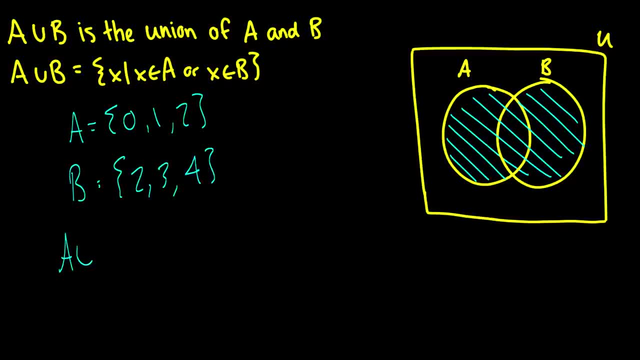 0 and 2, and let's take: B is equal to 0 and 2, and let's say Y is equal to 0 and 2, and let's say A is 2,, 3, 4, then A union B. we take everything in A and then we add everything in B. that is not. 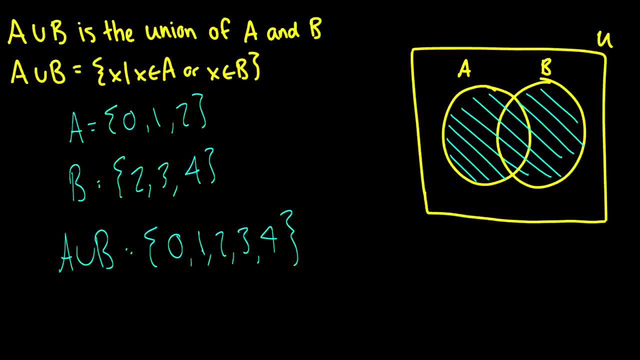 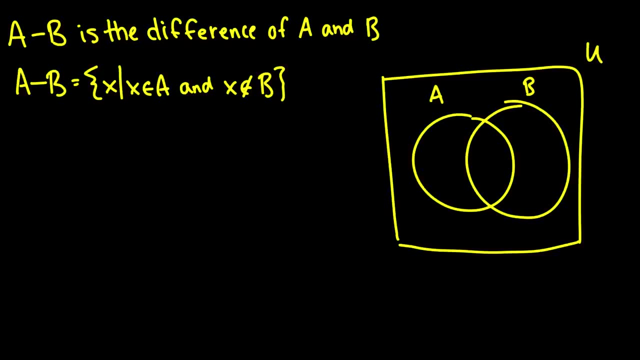 a repeat. So A union B is basically both sets combined into one set. We have one more operation here, which is the difference, and this is kind of what I was talking about with apples and stuff. This is A difference. B or A minus B is everything in A minus everything that is in B. 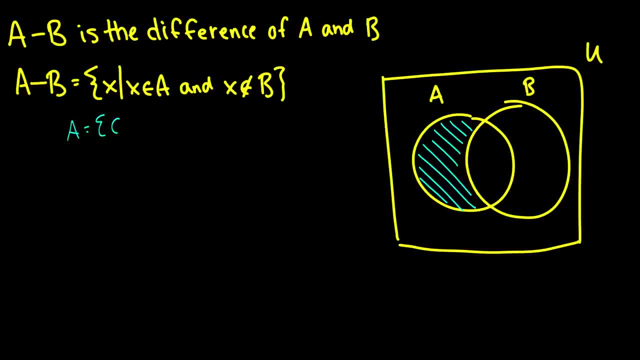 So if we take A is equal to 0,, 1,, 2,, B is equal to 2,, 3,, 4, then if we have A minus B, we take a look at the first element and we say, okay, we have 0.. Is 0 in B? No, it's not. 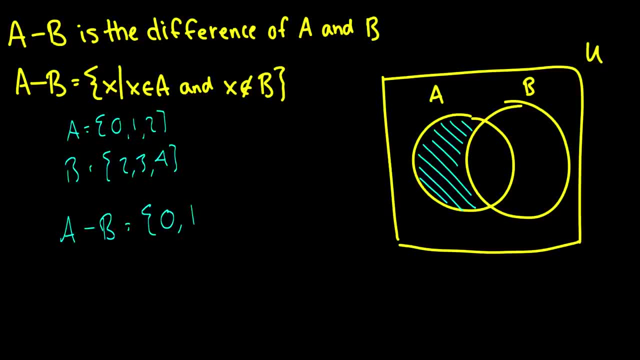 so we leave it in. 0 is 0 in B. 0 is 0 in B. 0 is 1 in B. No, it's not, so we leave it in. Now is 2 in B And we see that okay, yes. 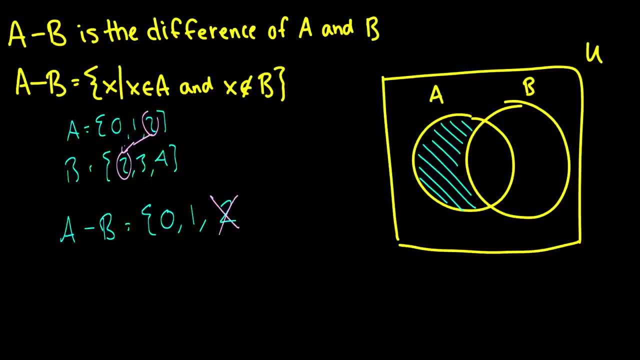 2 is in B, therefore we leave it out of the set, So it's not there. So that would be the difference set And, of course, if you have B minus A, in fact let's just write: uh, I wanted a different color for this. B minus A would be this: 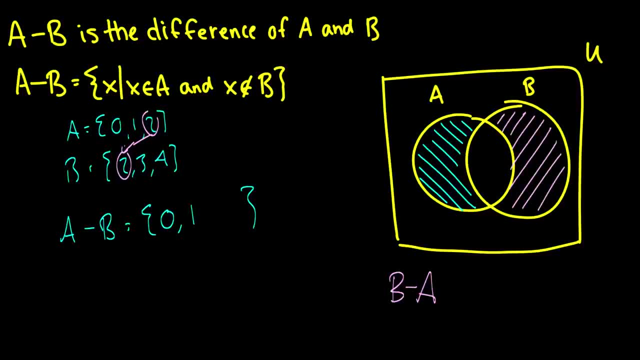 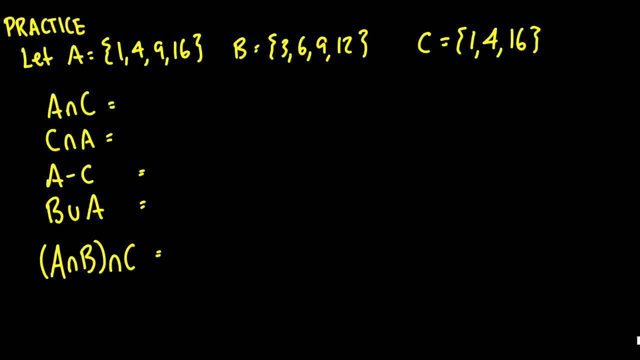 right here, All right time for some practice. We have A is the set 1,, 4,, 9,, 6,, which is the set of squares. We have B is the set 3,, 6,, 9,, 12,, which are the sets of numbers that increment by. 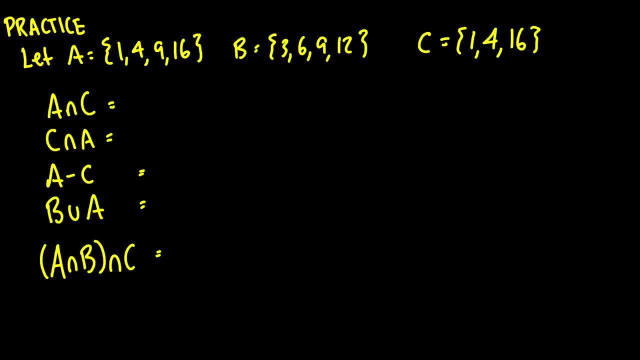 3. And we have C, which is 1,, 4, 16, which are some nice, not necessarily cubic numbers, but like 1 times 4 is 4,, 4 times 4 is 16.. I like these sets. They look. 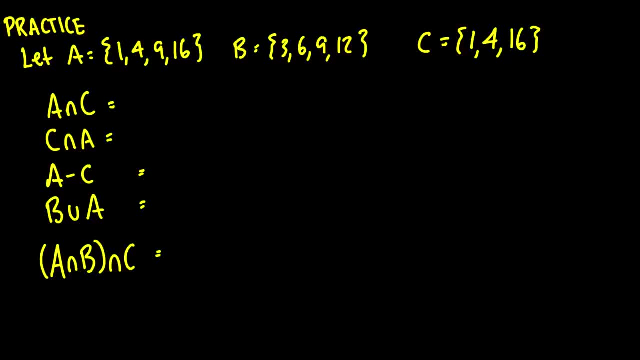 nice. Okay, let's take the union or the intersection of A and C. So we're looking at all the things in A that are also in C. So we see that 1 is in A and 1 is in C. 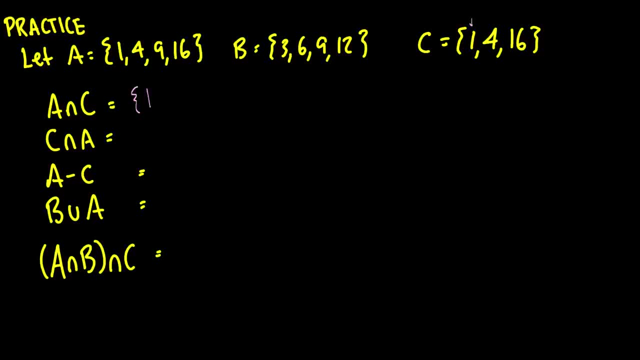 therefore, 1 is in the intersection. Okay, let's take a look at 4.. Well, 4 is in A and is 4 in C? Yes, it is, So we write 4 in our intersection set. What about 9?? 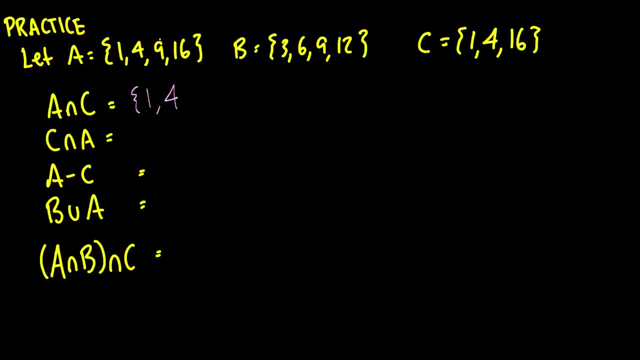 Is 9 in C? No, it's not, So we leave it out. And 16,? we see that 16 is also in C, So we include it, And what you'll notice is that A intersection C is actually just the set. 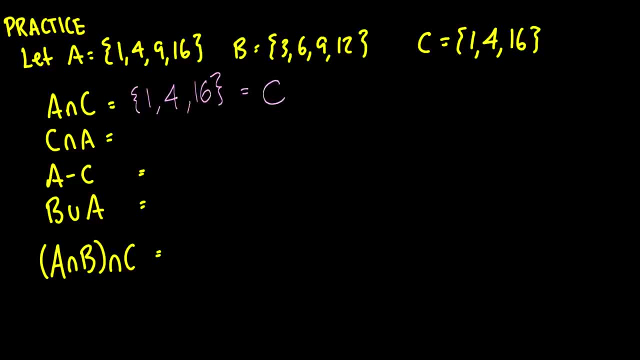 C itself, and this is because C is a subset of A. So if we take the intersection of something that happens to be in a subset relation, we're just going to get the smaller set out of it. Okay, what about if we reverse the order? Well, if we reverse the order, we actually get. 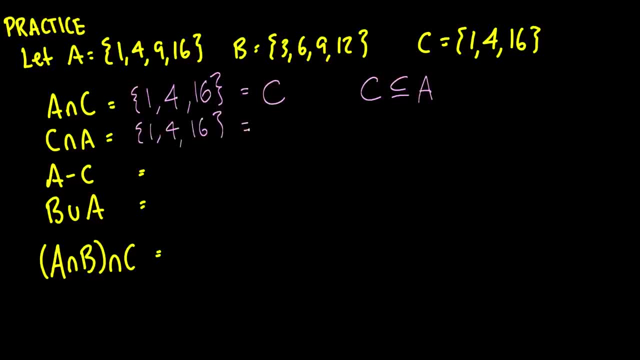 the exact same set, And this is an interesting property which we call commutivity. I'll just call it the commutative. I don't know if it's commutativity or commutivity, So it's the commutative. 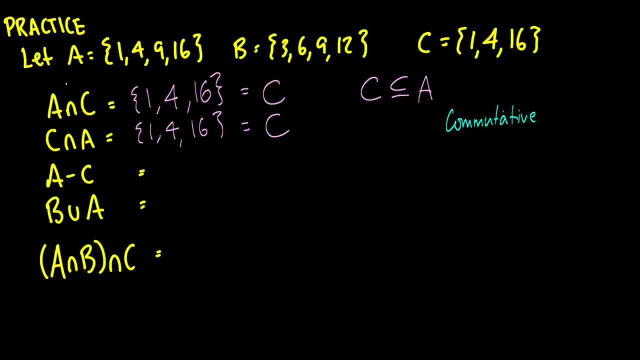 property, which means that we can change the order of our sets however we want, and it's not going to make a difference, provided we work with the same operator. So if we have, in this example down here we see B union A, then we can also have A union B. 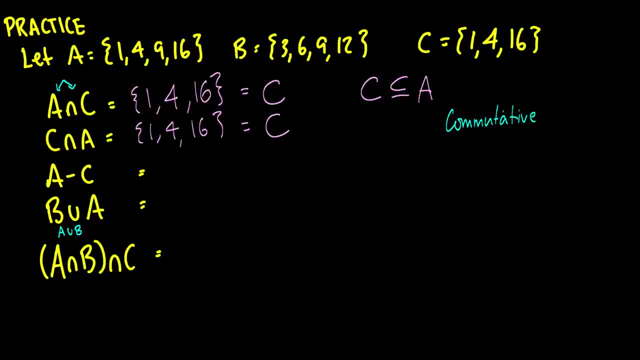 However, in this A minus C thing, we cannot do C minus A. This only works with the intersection and the union functions. Okay, let's do A minus C. Well, let's start with elements 1.. Is 1,? okay, so we have 1 in A. is 1 in C? Yes, it is, So we don't. 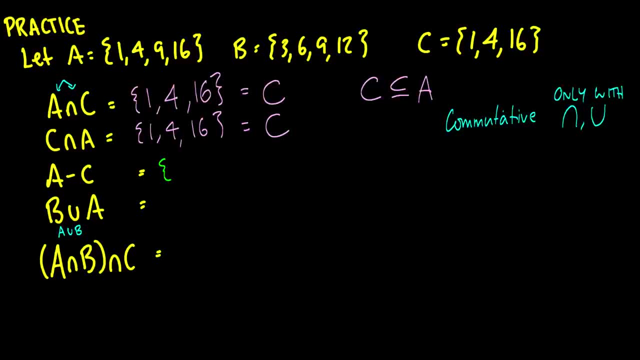 include it. What about 4?? Is 4 in C? Yes, it is, So we do not include it. What about 9?? Well, 9 isn't in C, so we include it, but we see that 16 is in C, so we don't include it. 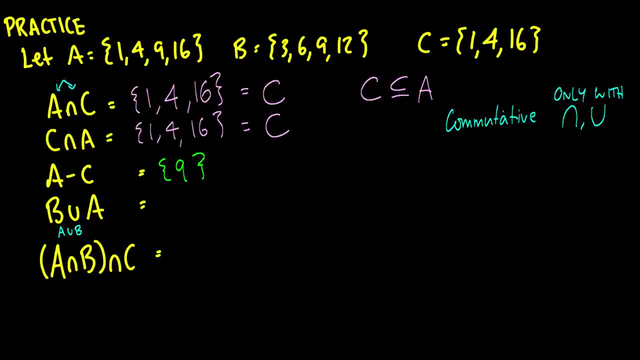 Now the interesting thing here is that if we have C as a subset of A, then this difference function is basically everything That's not in C, That is also in A, which I mean, is the definition. but it's interesting. 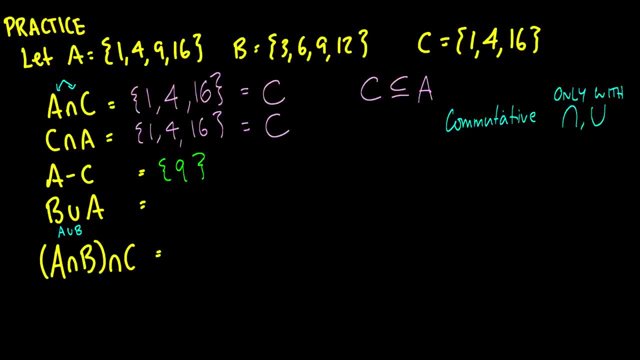 how, if we take- in fact this is a very good proof that you can eventually do- if we take C union, A minus C, then we just get A back, And I think that's something that isn't quite intuitive with notation, but if you think about this, 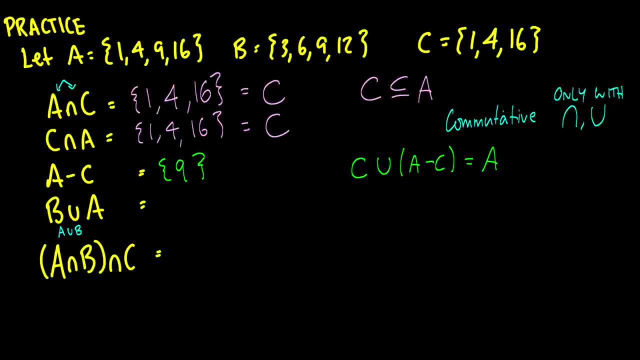 conceptually it's a lot more obvious and, I think, a little bit more intuitive. So play around with this kind of stuff. Eventually you'll be proving these things. Once we finish logic, talk about that a little bit more. we'll come back to set theory. talk about proofs. 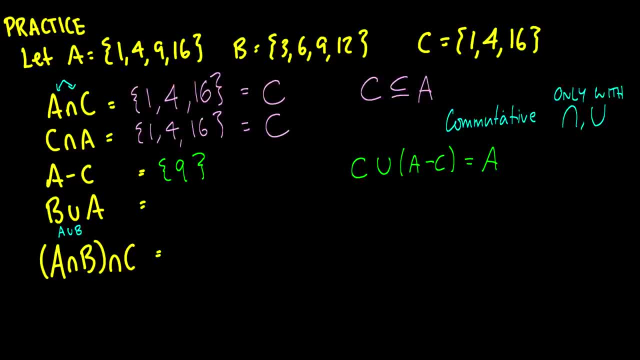 and we can prove this sort of stuff without examples. All right, B union A. Basically, what we do here is we take all the elements of A, All the elements of B first, It doesn't really matter- 3,, 6,, 9,, 12.. And then all the elements. 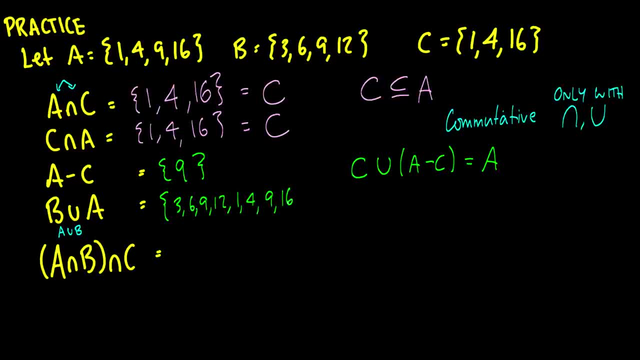 of A that are not repeated. Fortunately, we have none, so that would be the union. Okay, now, what we want to do here is we want to take the intersection of all three sets. So this is something that well. first of all, what you could do is you could take the 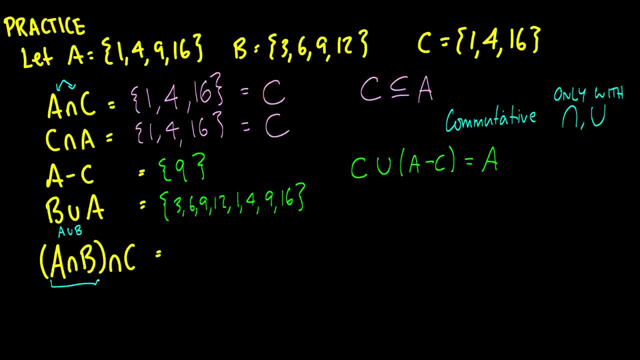 intersection of the first two sets, And I think that's what we'll do here. So what is A intersection B? What numbers do A and B have in common? I just noticed I included an element twice. Okay, so A and B, the only element. 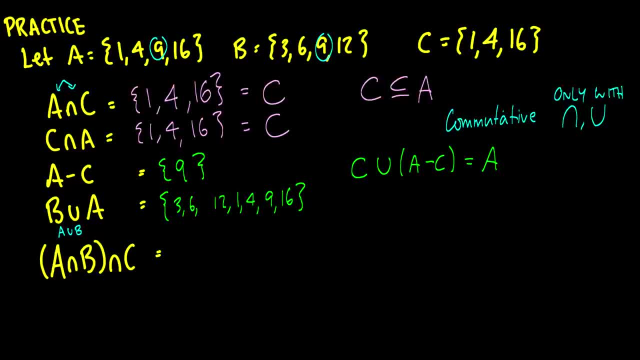 in common between the two sets are 9.. So we're going to have the set 9, and we're going to get the set 9 in C. No, it's not, So this final result is going to be the empty set. So what elements do? 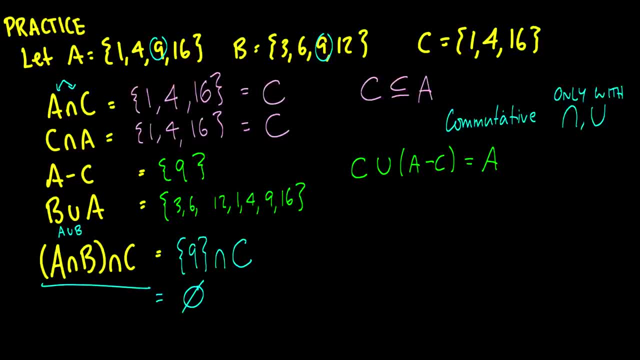 all three sets have in common? The answer is none. So that was some basic set theory practice with operations. That really I don't think was too bad. It definitely could have been worse. You'll probably see a couple more complex examples in your class And in the book.